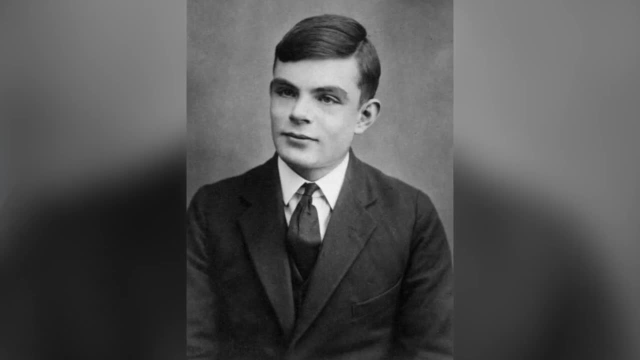 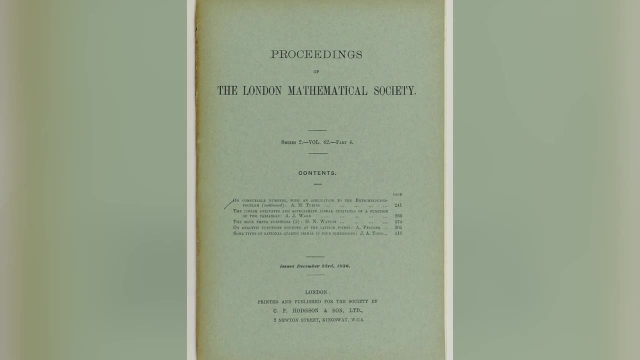 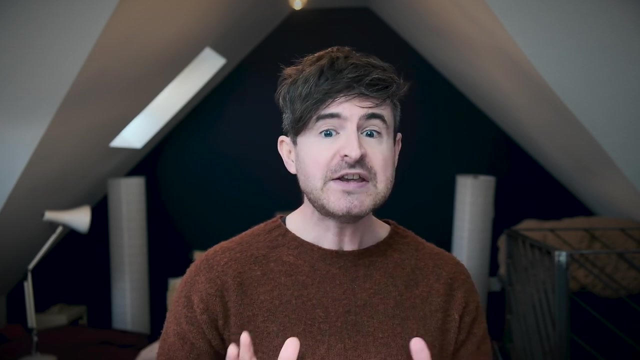 they got to do with the development of computer science. Okay, so let's talk about one of the main contributions that Turing made. It was in his paper on computable numbers, with an application to the n-shidings problem. Okay, so what is all of that and what did Turing do? So this goes back. 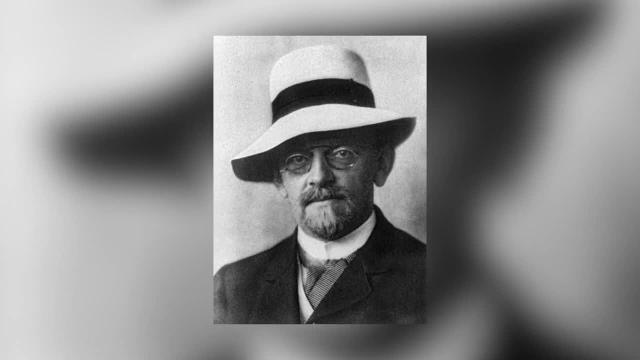 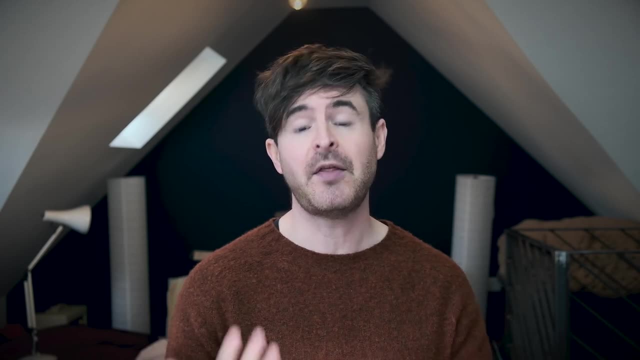 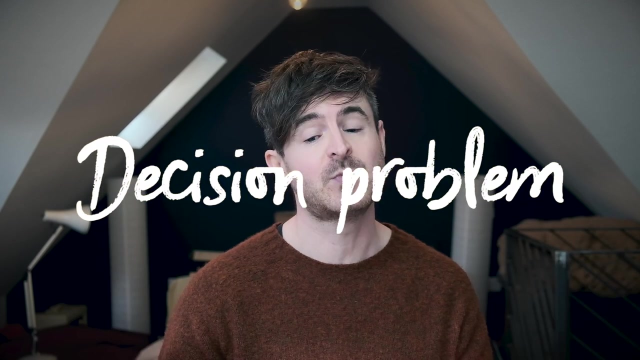 to the German mathematician David Hilbert, who at the turn of the century was the biggest mathematician in the world, the most famous mathematician- And he set out a number of problems or questions that other mathematicians would try to solve. In 1928, he posed the n-shidings problem, or the decision problem. So it goes like this: 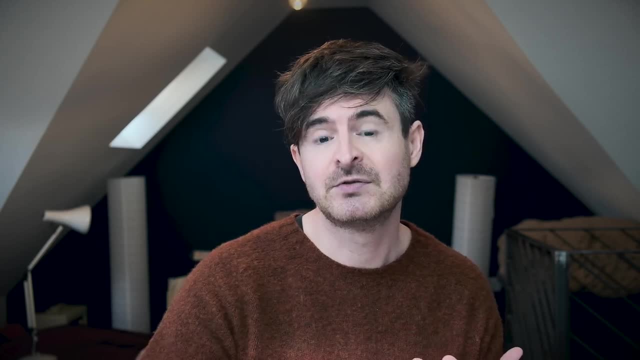 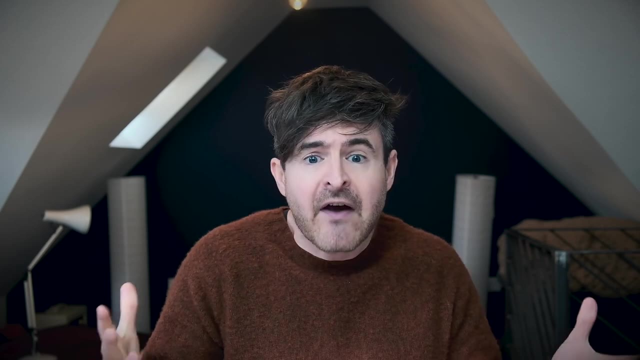 Is there an algorithm which, if you give it an arithmetical statement, it will give you a correct answer? Yep, that's true or no? that's false And because of various results in logic, that basically amounts to the question of: is there an algorithm that allows us to solve a problem? 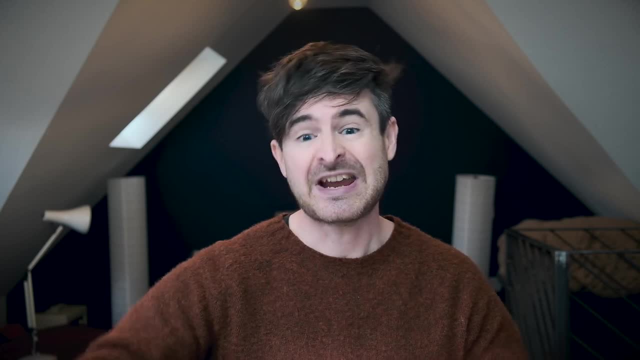 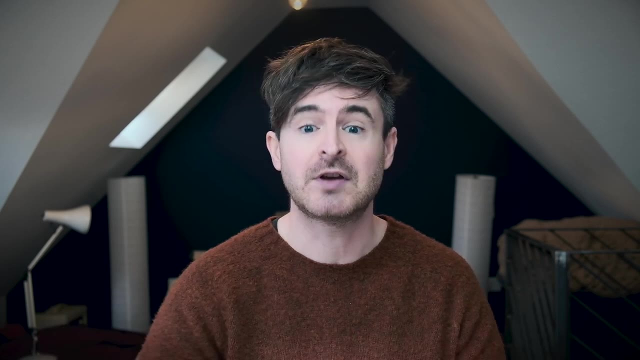 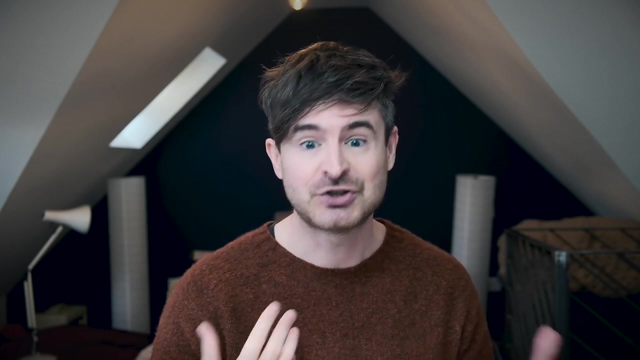 Is there an algorithm that allows us to deduce that answer from axioms of logic, if in fact it is an arithmetical truth? So if in fact it is deducible, can we automatically deduce it from the axioms of logic? Turns out, the answer's no, but it took real ingenuity on part of Turing to. 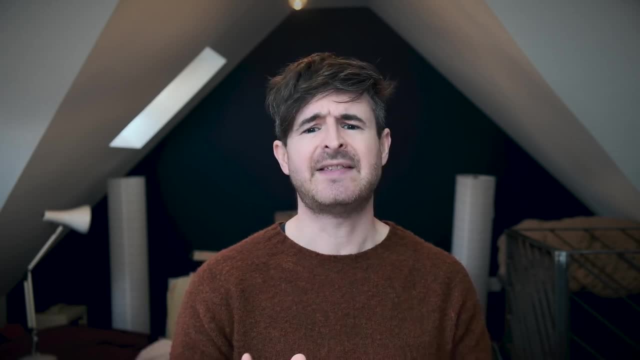 come up with that answer. So before we get on to how Turing did that, let's just spend a minute and think about why is that an important question? Well, we have to go back a bit to the turn of the 20th century, when mathematics theoretically was the most important thing in the world, And so we have to go back a bit to the turn of the 20th century, when mathematics theoretically was the most important thing in the world. And so we have to go back a bit to the turn of the 20th century when mathematics theoretically was the most important thing in the world, And so 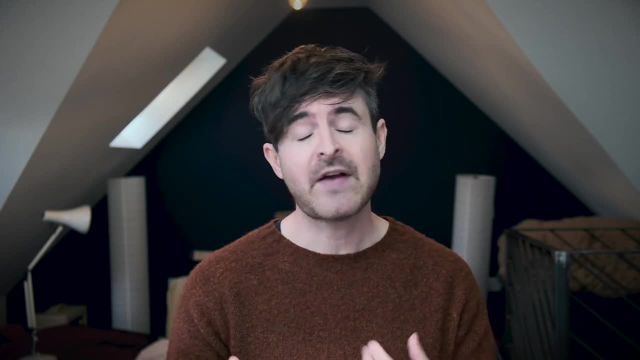 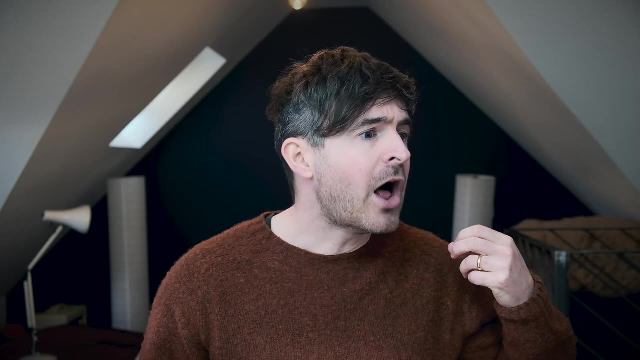 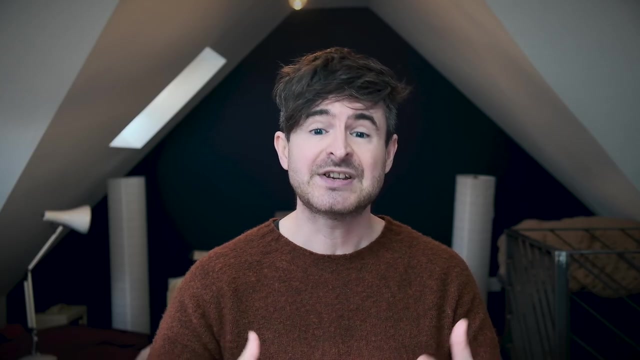 mathematical mathematics was in kind of a little bit of turmoil. People had found lots of paradoxes. There was this general feeling that the foundations of mathematics wasn't on good footing And a lot of mathematicians and philosophers, so people like the German Frege and Bertrand Russell. they were trying to establish mathematics on sound footing by 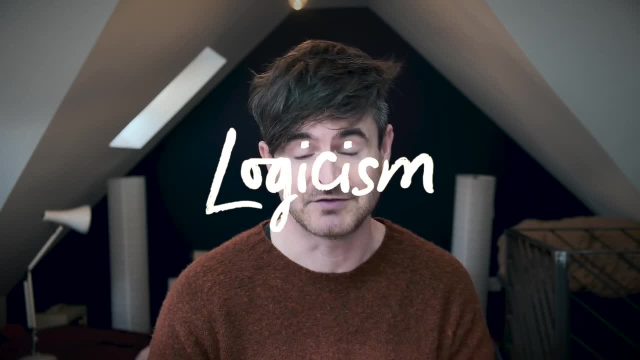 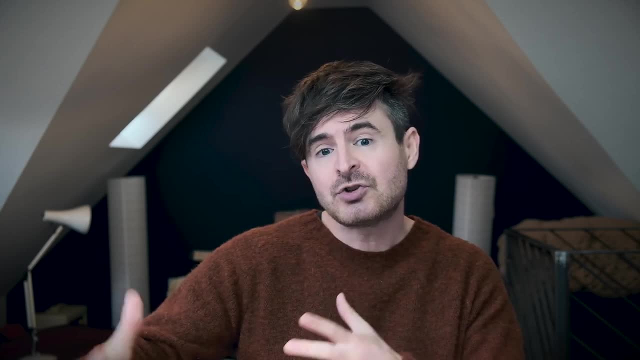 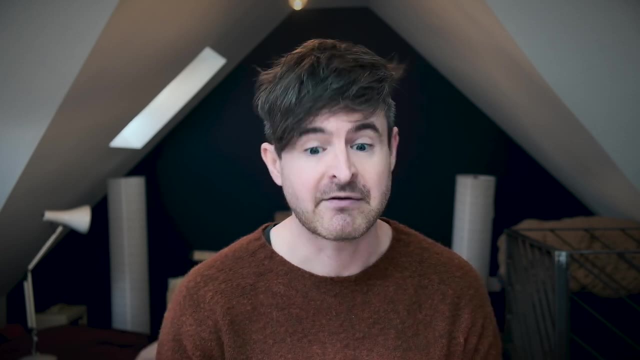 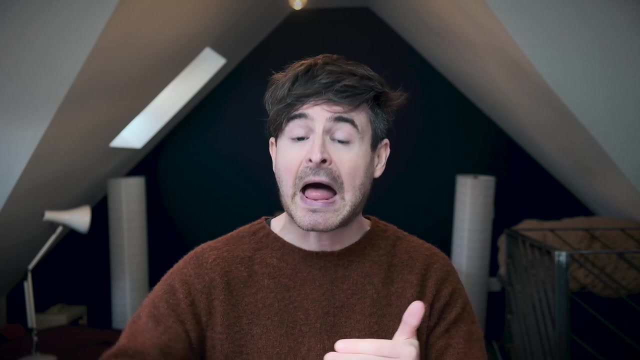 We do logical proofs. So if we could transform mathematics into this purely logical procedure, then we could avoid all the paradoxes. Okay, but in order to do that, we first needed to know just how much of this careful, algorithmic, logical reasoning could we do. okay, So this is where the 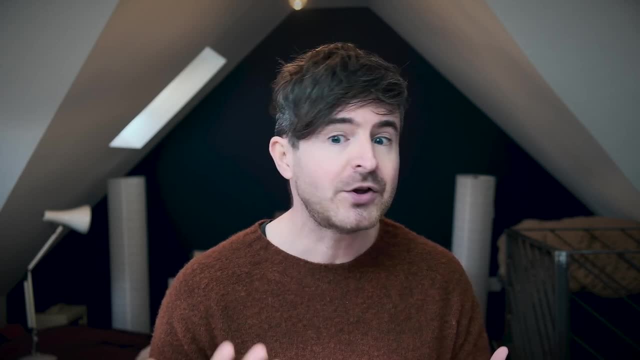 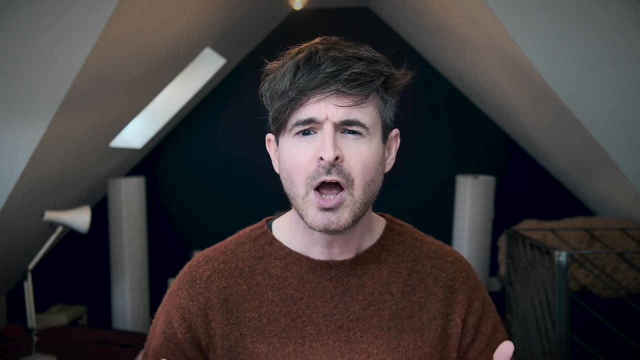 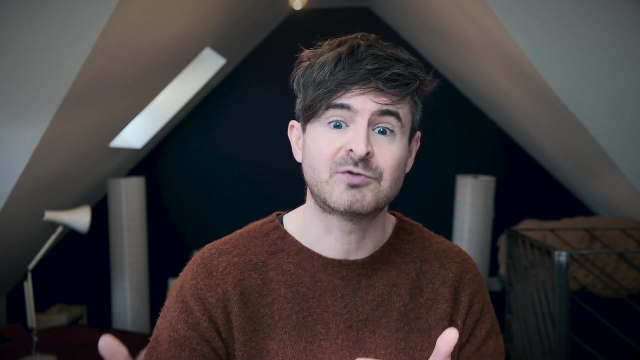 decision problem comes in. Just how possible is it to derive truths of mathematics, truths of arithmetic, from the axioms of logic? Not by guesswork or intuition, but just by using an automatic algorithm. okay, So that's why the decision problem was important. Okay, so when? 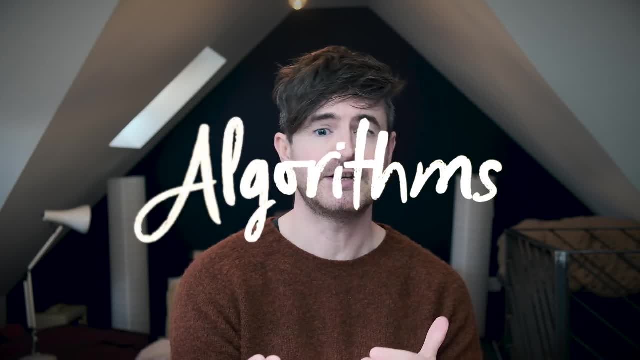 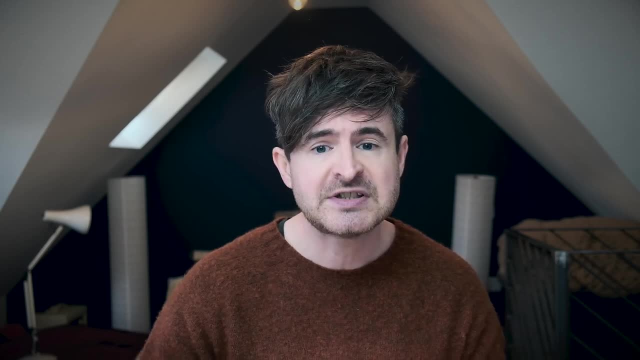 we're thinking about an algorithm here. we're thinking about an automatic procedure that follows a definite set of instructions. So if you are following that algorithm, you don't have to use any ingenuity or intuition or understanding even You just follow the instructions and you. 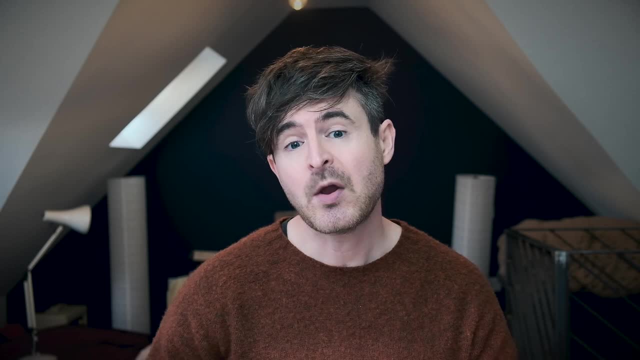 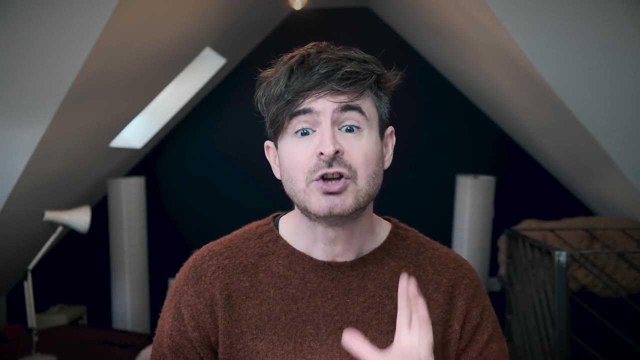 take an input and you do some stuff and you give an output. So that's why they wanted the existence of algorithms for solving problems in logic and mathematics. So Turing showed us that no, there isn't always an algorithm, There isn't always a. 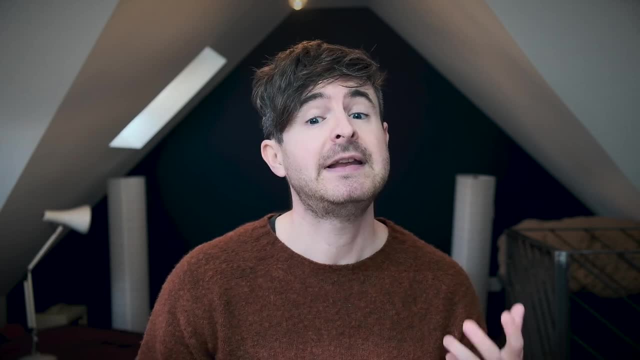 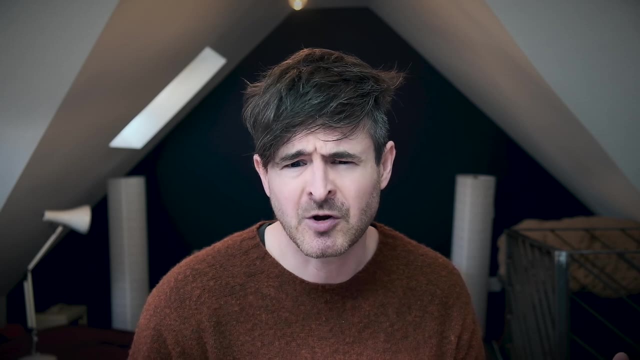 solution to the decision problem. Now, Turing gave himself a really difficult task here, right, Because he's trying to show that there is no possible algorithm that solves a particular problem. How do you do that? How do you show that no algorithm can do it If you're arguing the other? 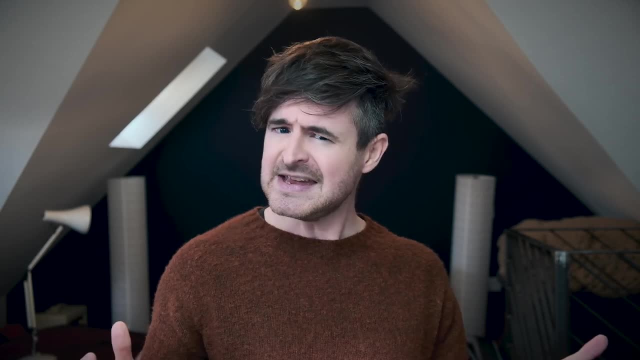 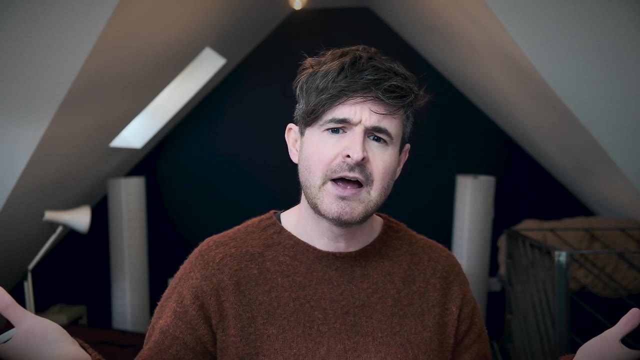 way and you want to show that, yeah, there is an algorithm that does it. It's kind of easier. You just provide the algorithm. So if I give you an algorithm that does something, I have proved that the algorithm exists, But if I want to prove that no such. 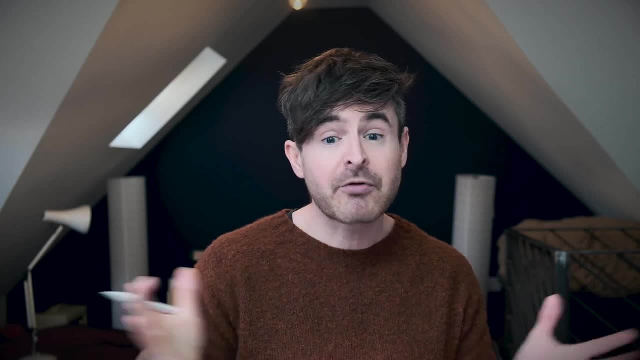 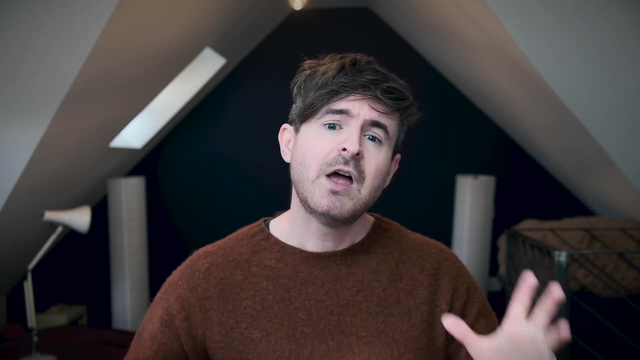 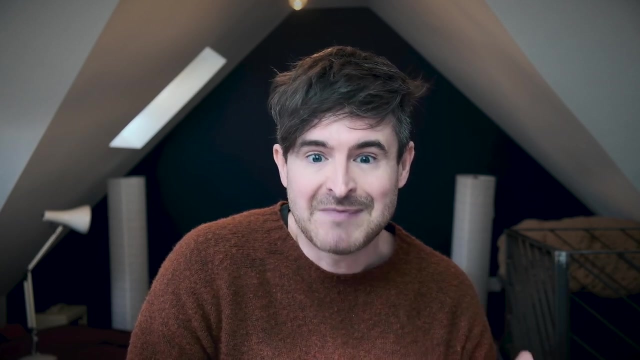 algorithm exists. how on earth could I do that? It's not like I can go through every single algorithm, because there's infinitely many of them. Turing came up with a really, really clever argument, So the first step was to basically make the notion of an algorithm official mathematical. 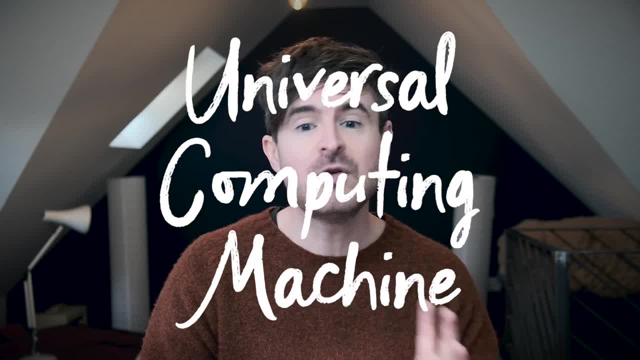 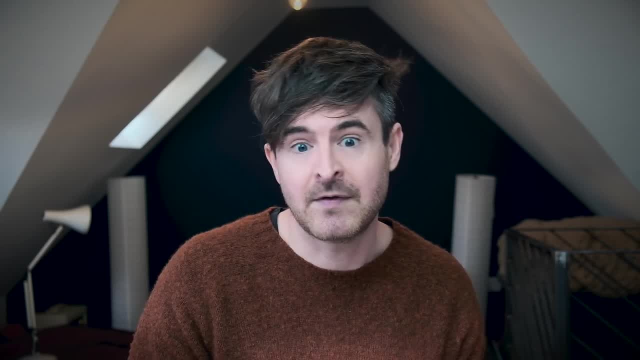 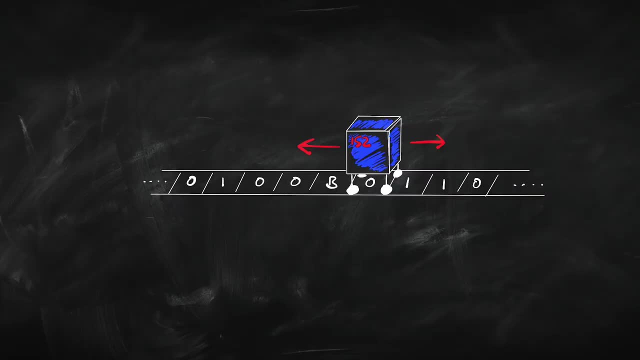 formal. He came up with the idea of what he called a universal computing machine, a machine that he described mathematically, that could do anything that any algorithm could do. Okay, This is the notion of a Turing machine. So let me describe that for you right now. A Turing machine is: 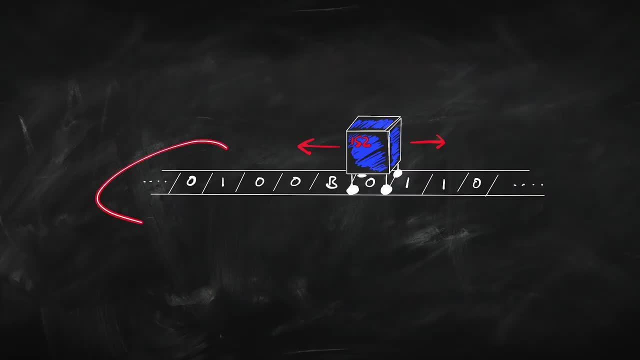 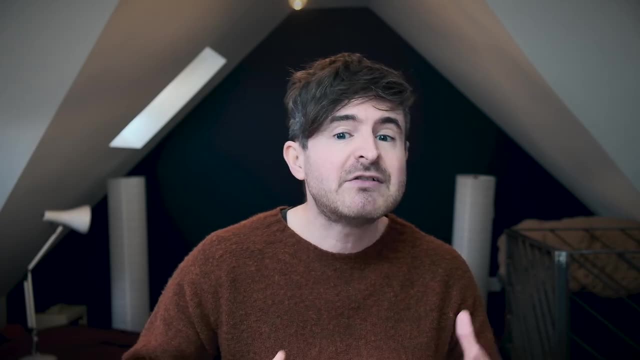 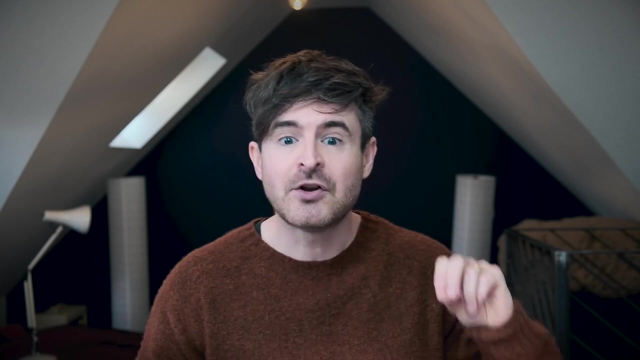 basically something like this: So we've got a tape. On the tape we have ones and zeros written, and we might also have some spaces or some Bs for blanks, And the idea there is: we can code any problem in mathematics in binary strings of ones and zeros. Then we've got something that is going to read symbols on this. 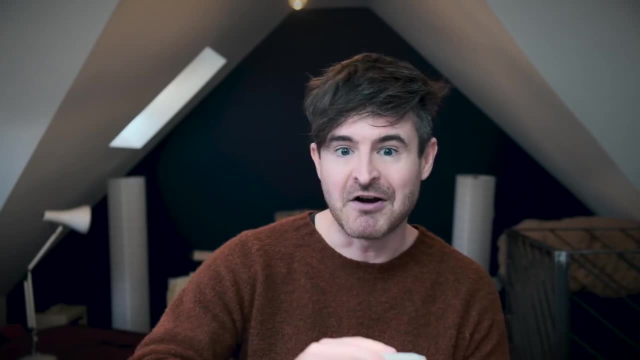 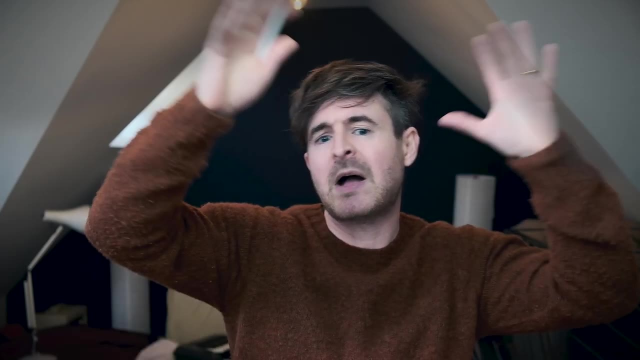 tape one square at a time. So this little box here it's going to run up and down the tape and it's going to look at one square at a time And it's got a state. And you can just think of that as a number, like: imagine a big wheel with all numbers around it And that records what state. 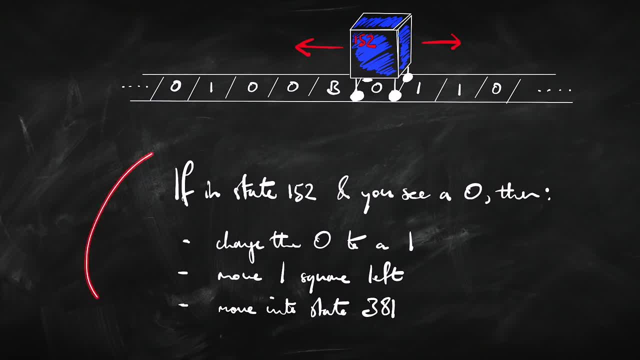 this machine's in, Okay. So what does this machine do? It has a program And the program has a number of instructions in it, And they're basically super simple. They say things like this: If you're going to do something, you're going to have to do something. If you're going to do something, 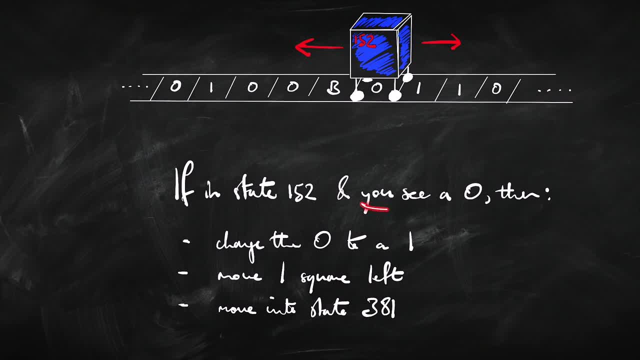 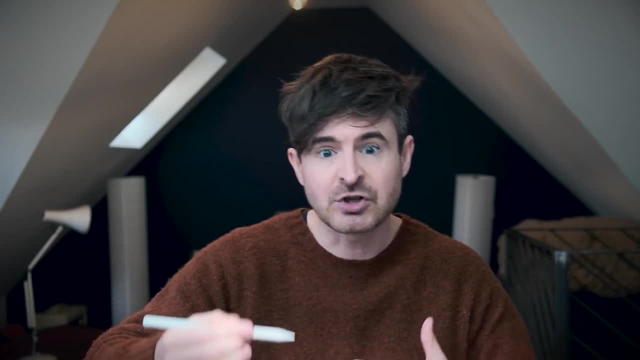 you're going to have to do something. If you're going to do something, you're going to have to do something. If you're in state number 152, and you're looking at a zero, then do the following things: Maybe you're going to change the zero to a one, So the Turing machine it can rub out and write new. 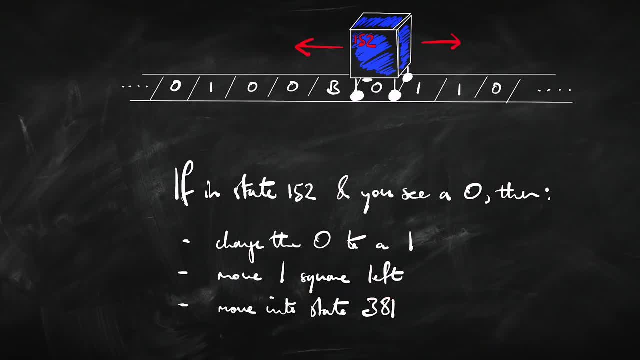 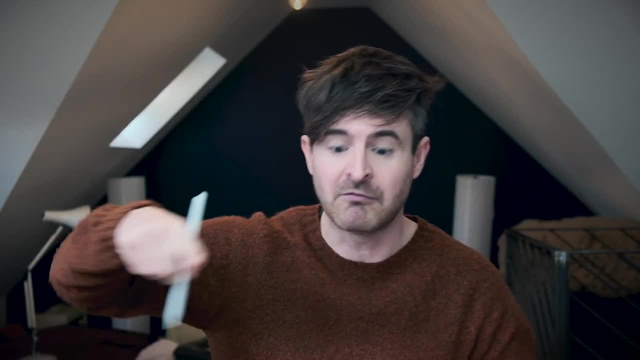 symbols on the tape, It can move. It can move left or it can move right, And then it can move into a new state. Okay, So if we imagine this state as a big wheel with counters on it, you basically just kind of move the wheel around until you're in state number 381, or whatever. Super, super simple. 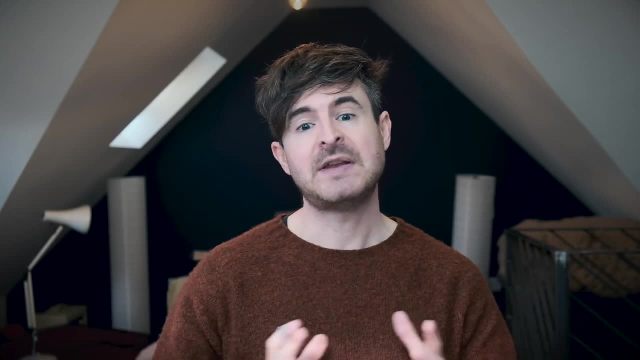 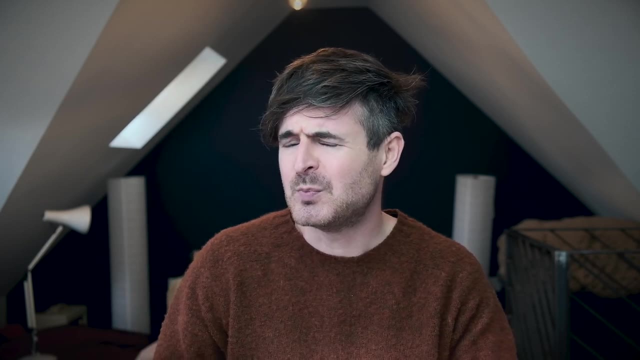 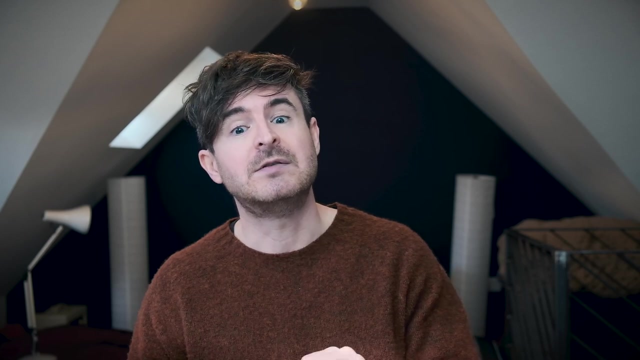 But Turing's idea was: anything that can be done by any algorithm can be done by a machine like this, by a Turing machine. Now, that's not something you can prove, So that's called the Church-Turing hypothesis. Anything that can be computed can be computed by a Turing machine, Pretty much. 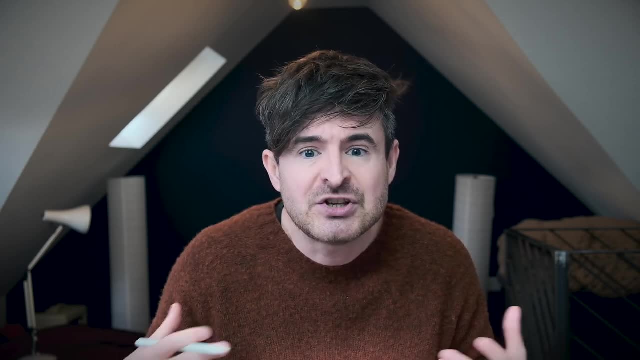 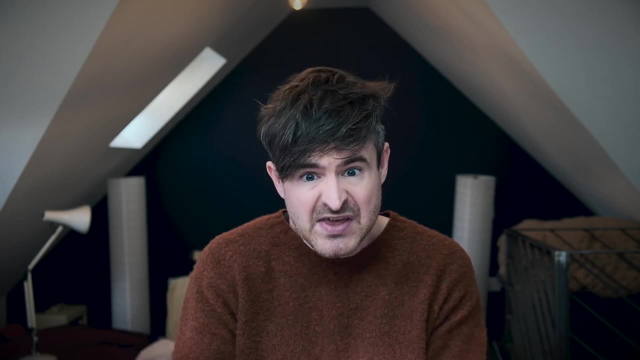 everyone believes that that's true. The notion of computation is kind of informal. There isn't an exact definition. You can think of this as a definition of computation- Okay, This is what the Turing machine's doing, That is what computation is. And then it becomes not just a. 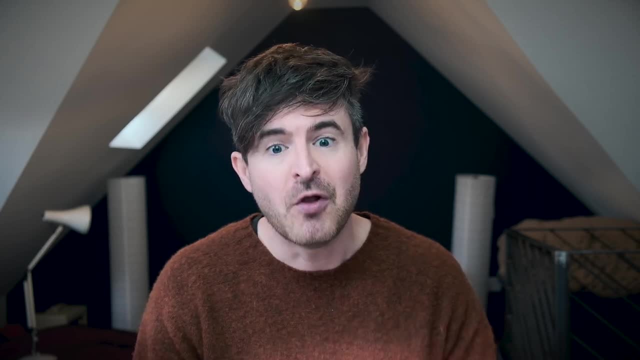 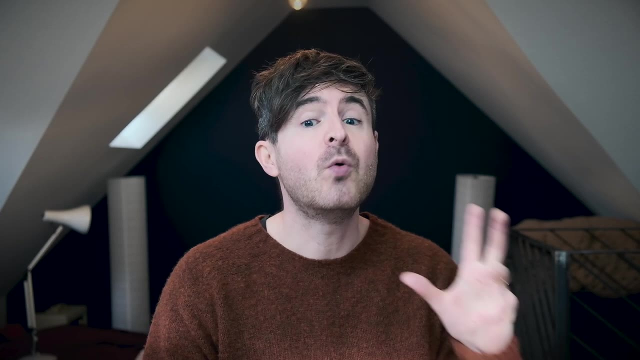 hypothesis, but a theorem. So how would Turing show that no Turing machine could solve the decision problem? Okay, That's what he's trying to do. He's trying to show that no algorithm can solve it by showing that no Turing machine can do it. Because if an algorithm could do it, 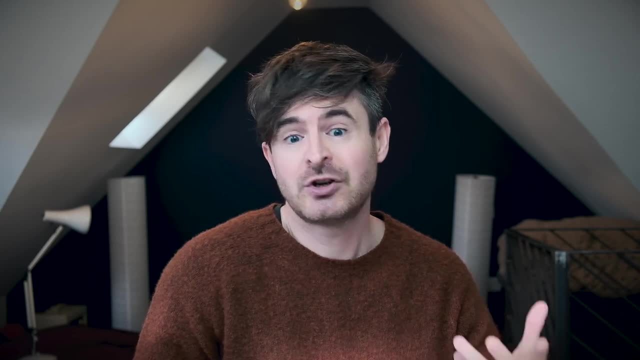 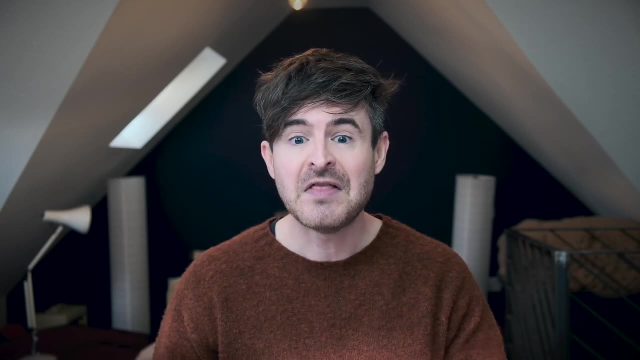 a Turing machine could do it. First of all, he showed that a Turing machine can't solve another problem- It's called the halting problem And we're going to get to the that in a bit. And then he showed that, well, if you can solve the decision problem, then you can. 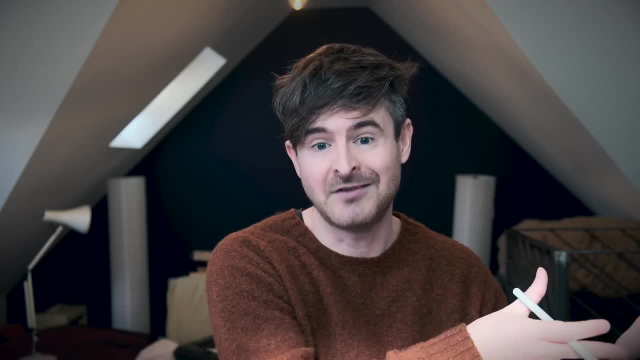 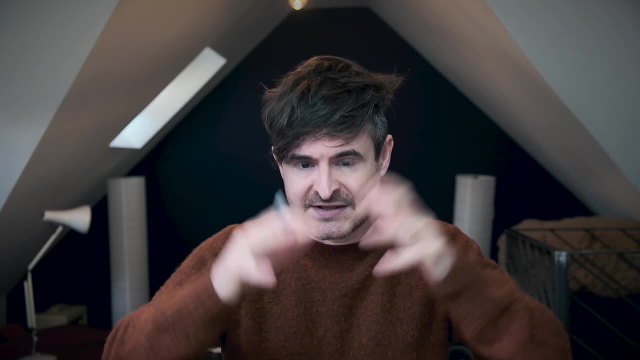 solve the halting problem. but you can't solve that, So you can't solve the decision problem, The halting problem. it's really cool, Okay. So let's have a look at it. We've got all these Turing machines right. We're going to take a Turing machine with its program and we're going 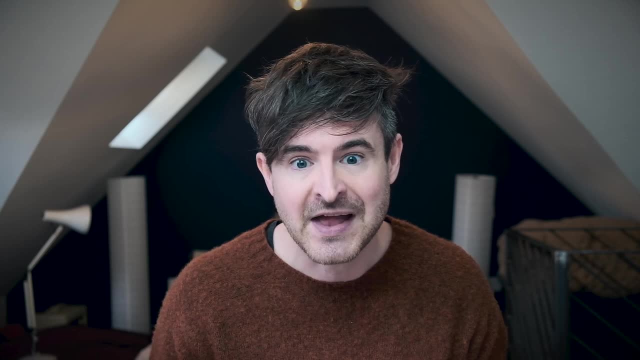 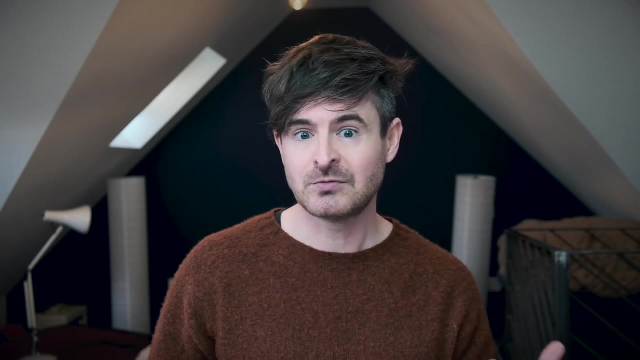 to put a tape into it And the Turing machine is going to do some stuff with that tape And the output will be whatever's written on the tape when the machine halts. So Turing machines, they have a special state. Just think of that as the halting state. And if they 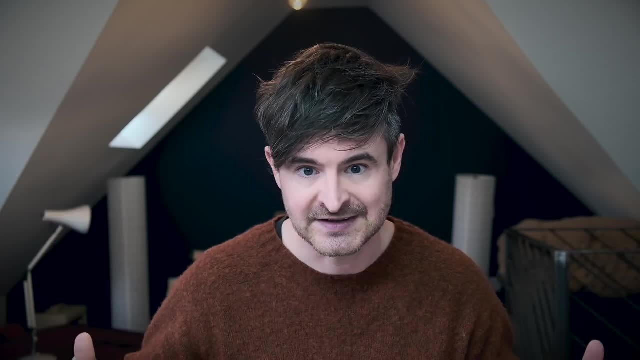 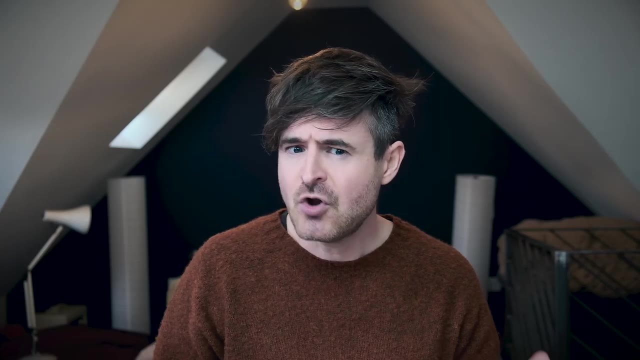 get to that state, it stops. And then we say it's halted. A machine won't always get to that state. Okay, A machine might halt, but it might not halt. How could a machine not halt? Well, suppose it had a really daft program like this. Okay, You've got these two instructions. 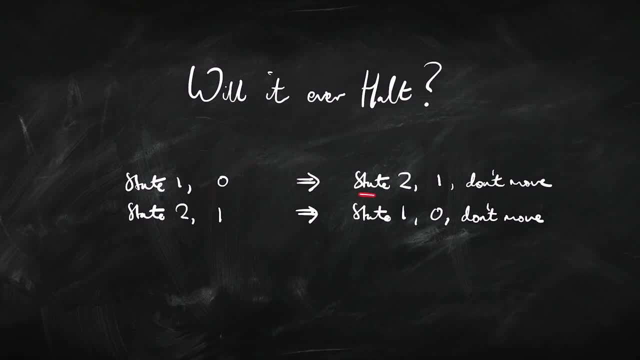 If you're in state one and you see a zero, then go into state two and write a one there. If you're state two and you see a one, then go into state one and write a zero there. Okay, That's a pretty. 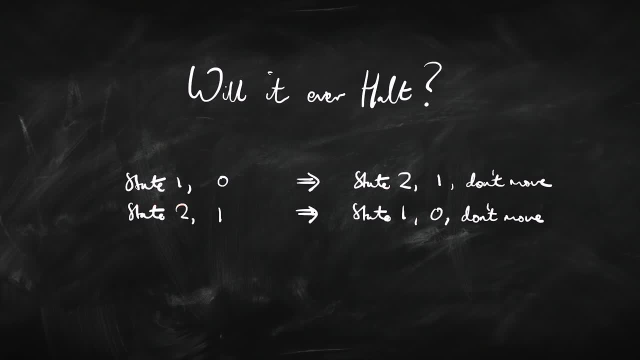 daft program, because if you do end up in this state, then you're going to go into this state, And then you're going to come back here, and you're going to go into this state, And then you're going to go back here, and these instructions will just loop around forever. Okay, So if you get, 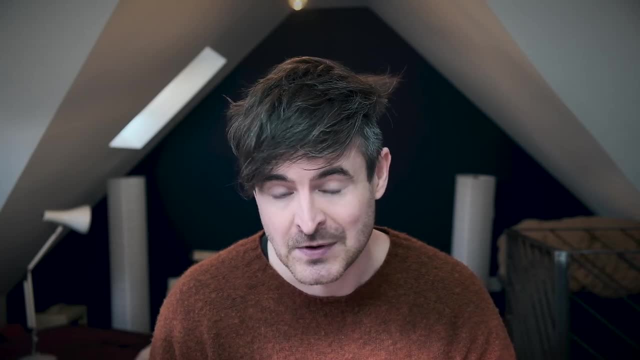 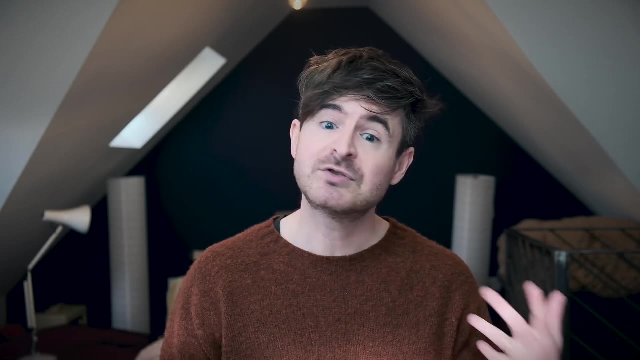 caught in this loop here, you're never going to get to the halting state. So a program like this, if it does see a zero in state one, it'll just loop forever and it won't halt. So sometimes a particular Turing machine with a particular program, with a particular 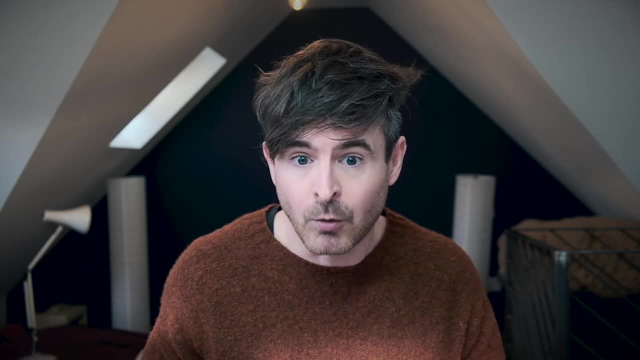 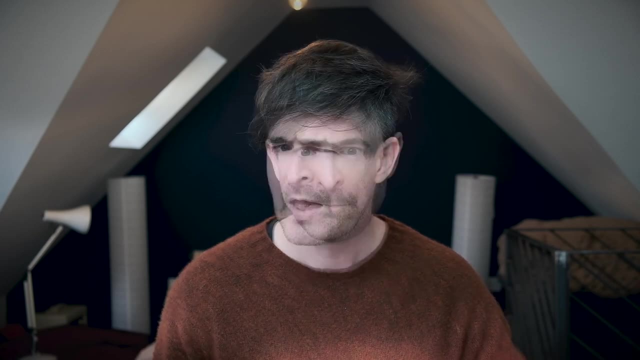 string on the tape, it won't ever halt. Some machines will halt if they get a certain input Okay. So it'd be nice to know if we're going to give this input to this Turing machine, is it going to halt or not? How could we tell that? Well, we could run it and see. Maybe it. 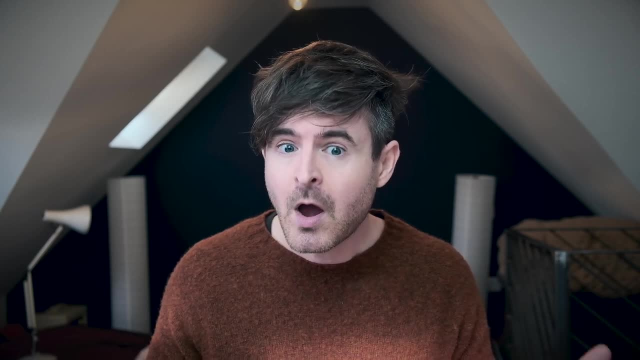 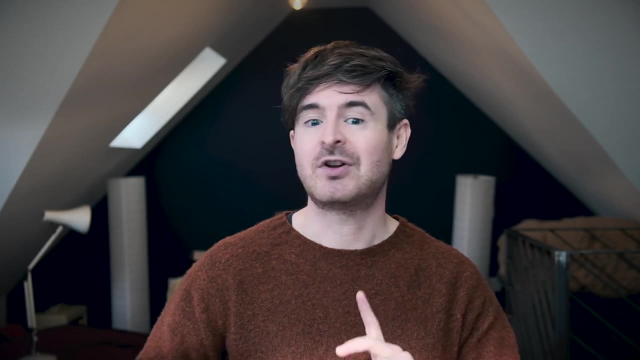 takes too long. It'd be nice to be able to kind of work it out with an algorithm. Oh, an algorithm, That's what Turing machines do. So it would be nice to have a Turing machine that can tell us if I've got this Turing machine over here and I put this tape into it. 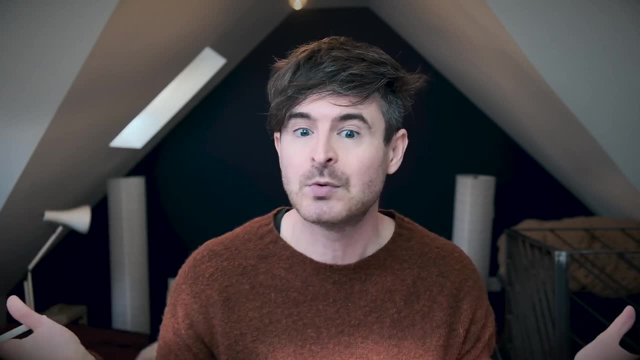 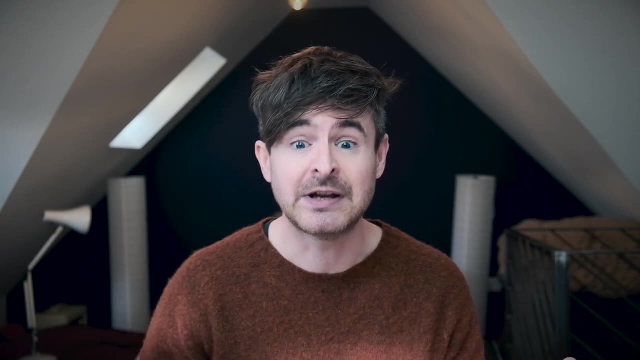 is it ever going to halt or not? Could I have a Turing machine that will tell me that Turing proved that there can be no such machine because basically it would be contradictory, And his argument for that is really, really, really cool. So let's have a look at how it goes. 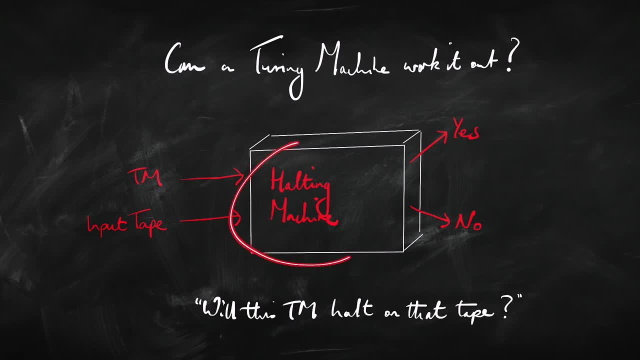 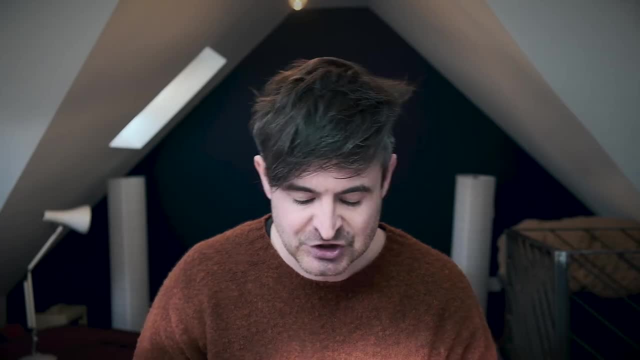 Let's suppose we did have such a machine. Okay, So let's suppose that we've got this machine. Don't care about how it works. Let's suppose it's magical or whatever. Let's just imagine that there exists this machine And what we're going to do is we're going to feed it with information about a. 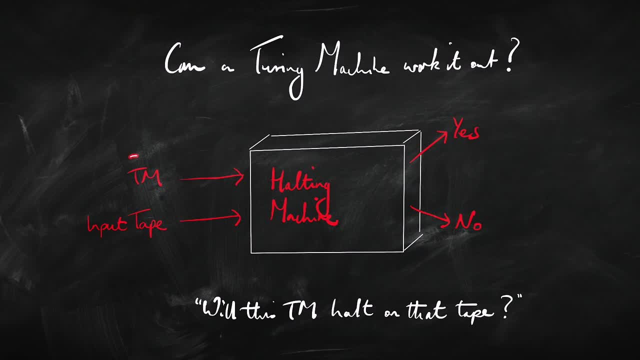 Turing machine and an input And we ask it a question: Is that Turing machine going to halt with that input? Basically, what we're doing is we're taking the Turing machine, we're coding it up on a tape and then we're sticking this input tape at the end of that tape and we're putting 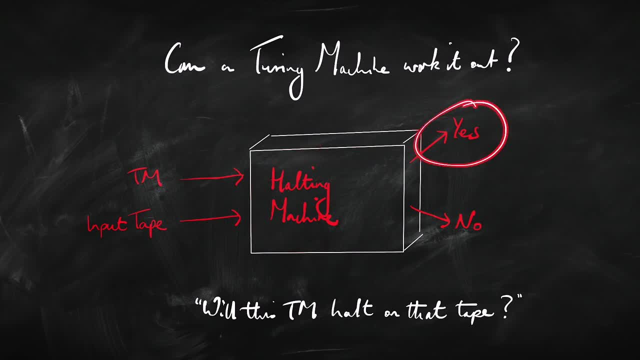 it all into the halting machine And we're going to get an answer: Yes, that machine's going to halt, or no, that machine's not going to halt. Turing then gave a really nice argument that shows that this little box here is impossible, And it goes like this: Well, if that machine is, 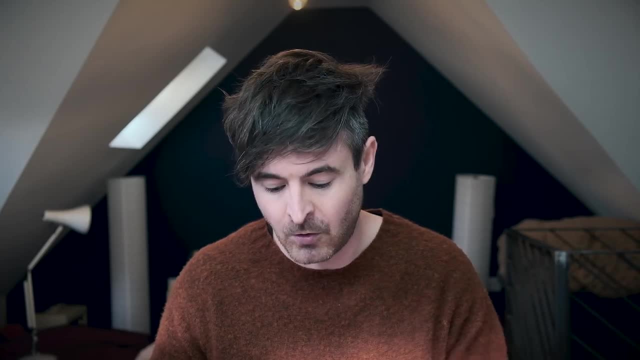 possible, then it's going to halt. And if that machine is impossible, then it's going to halt. Then we can fiddle about with it and add a bit more and end up with something like this. So what we do is we take a little machine that just goes around in a loop, like the program we talked about. 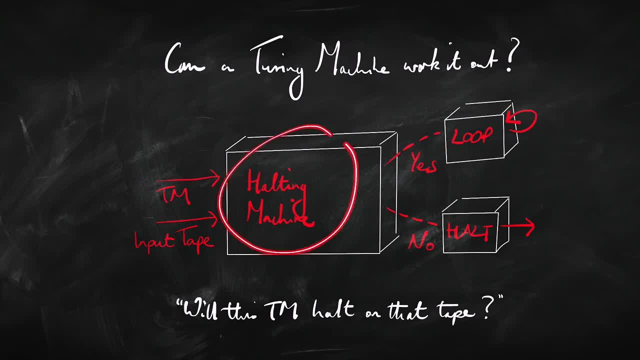 a minute ago and we connect it up to the yes output. So if this machine answers yes, we go into this machine. okay, and we just loop forever. And then we connect up the no output to a machine that basically does nothing apart from halting, So it just basically jumps straight to the halt. 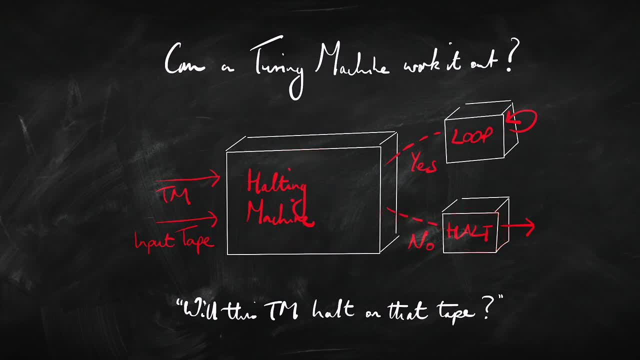 state: So if this machine answers no, then we just halt straight away. Obviously, if that machine exists, these machines exist, so the whole thing exists. Okay. so if that's possible, then all of that big machine is possible. Here's the problem. Suppose we code up the whole machine, this whole. 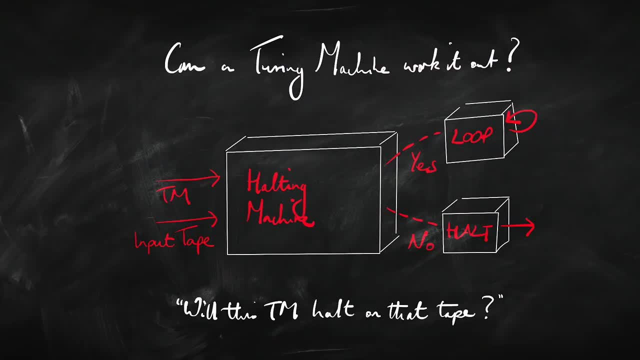 great big thing here. we write that description down on a tape and we feed that tape in here. So we basically feed a description of this machine into itself And we say, okay, we give you some input. are you going to halt or not? What's the machine going to do? Well, if it is going to halt, 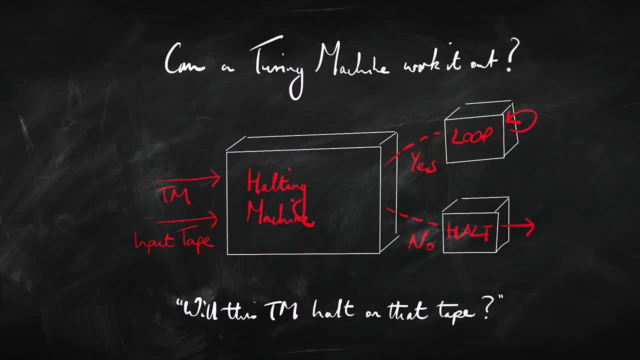 this machine will say yes, Then we go into a loop so we don't halt. So if the machine would halt, it wouldn't halt. Okay, so maybe it's not going to halt, But if the machine doesn't halt, this part of it answers no and we 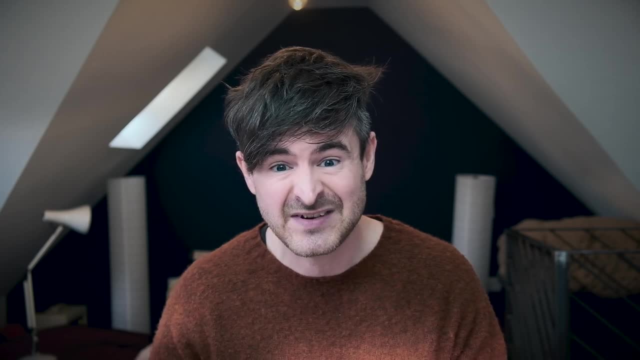 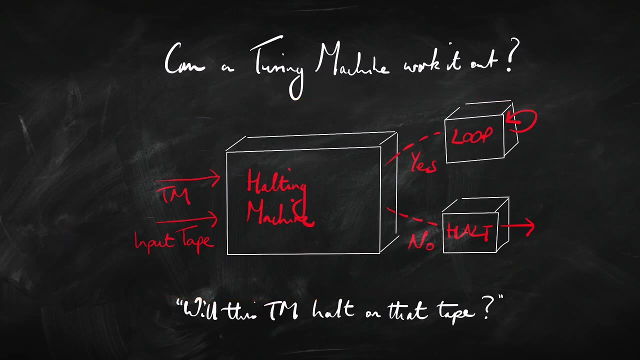 go into this bit and it does halt. So if it doesn't halt, it does halt, And if it does halt, it doesn't halt. It's a contradiction. either way, This machine is impossible. It's contradictory. And because this thing is contradictory, but these bits are possible, it's this bit that's the problem. The. 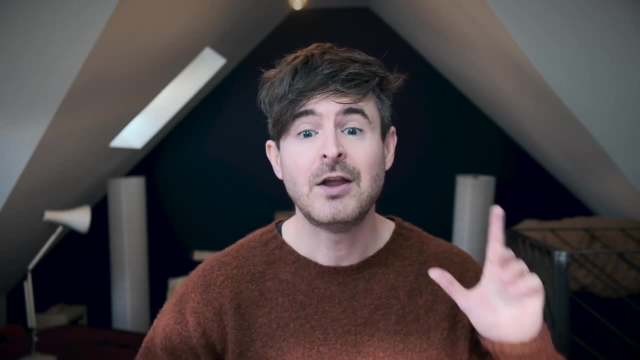 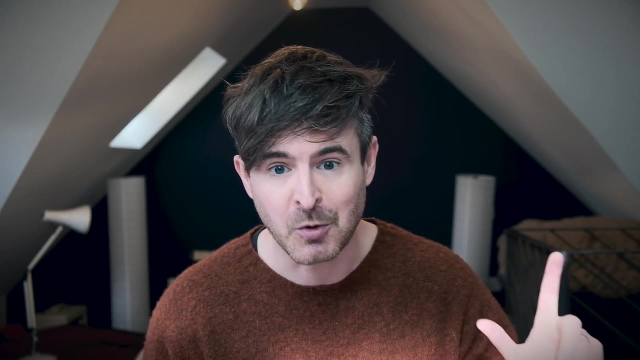 machine is impossible. It's impossible, It's contradictory. No Turing machine, no algorithm can solve the halting problem. Okay, that's super important, That's a really important result, because it comes up right the way through computer science. So the halting machine is impossible. 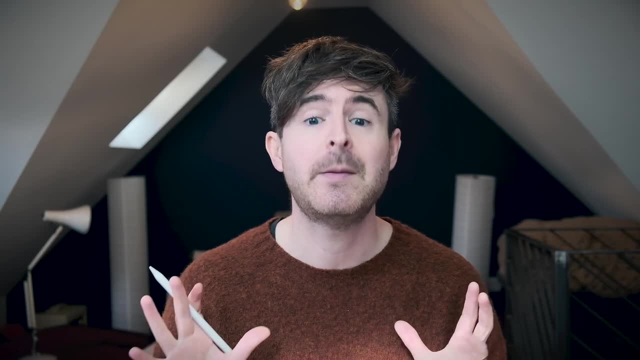 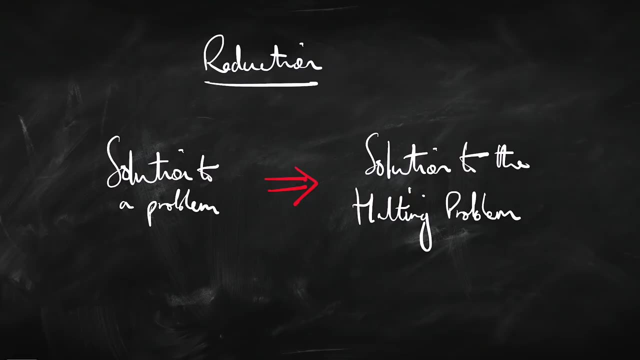 The halting problem is undecidable. That is a super important result and it comes up right the way through theoretical computer science. Here's how it gets used. Suppose you've got some problem you're interested in. You've got a problem that you're interested in. You've got a problem that? 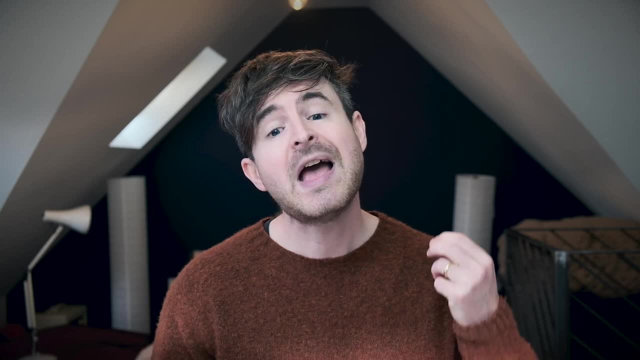 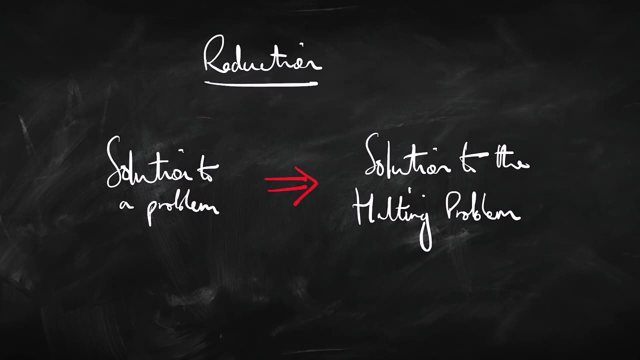 you're interested in Okay, and you want to show: is it solvable or not? Well, here's a way that you can show that it's not solvable: You use what's called reduction. You reduce your problem to the halting. 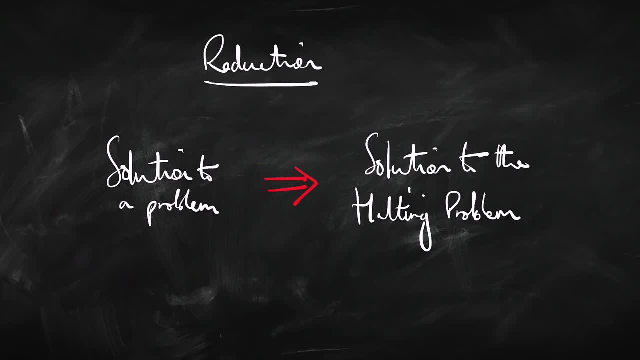 problem. So you show that if there is a solution to your problem, then there would be a solution to the halting problem. but there isn't a solution to the halting problem, so there's no solution to your problem. That's a general strategy that computer scientists use all the time, every day. 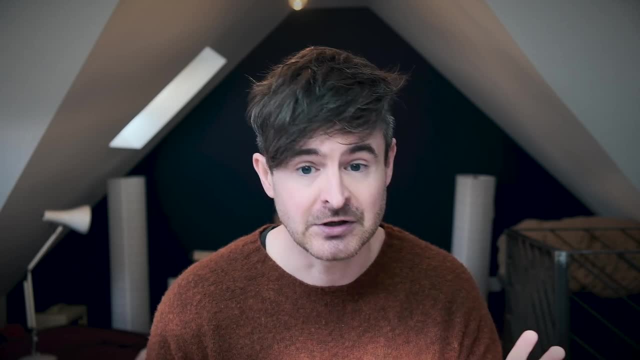 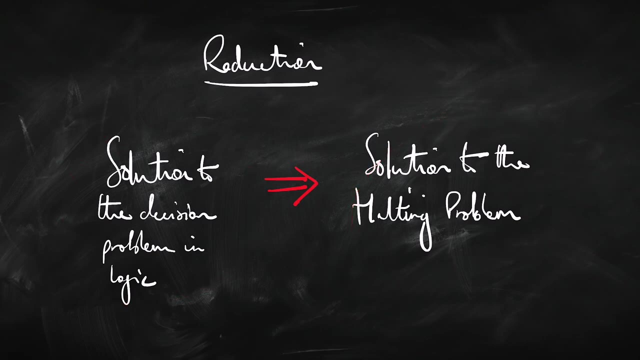 Here's how Turing used it to show that there's no solution to the decision problem. He basically said: yeah, look, if there is a solution to the decision problem, then we can solve the halting problem. but we can't solve the halting problem, so we can't solve the decision problem. So all he needed then is: 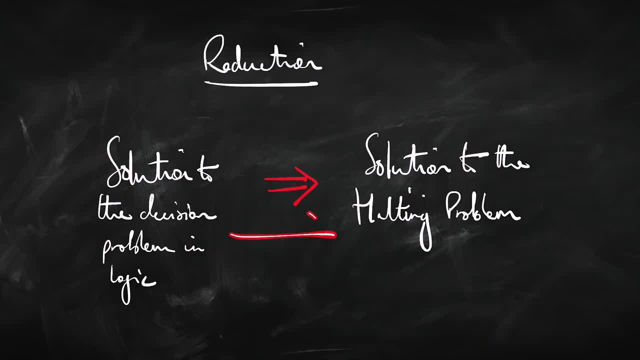 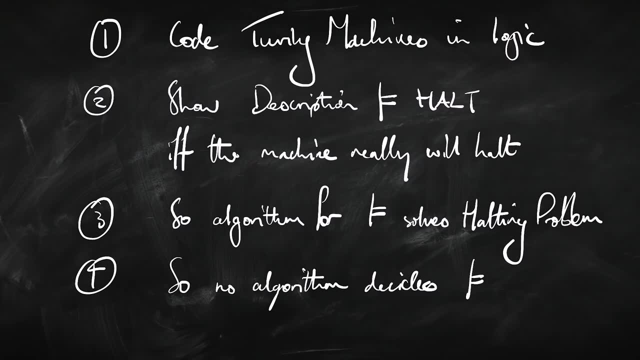 just a little bit more argument to show that this bit. basically, if you can solve the decision problem, then you've already solved the halting problem. He had a really nice argument for that and it goes like this: So we can code up Turing machines in logic.